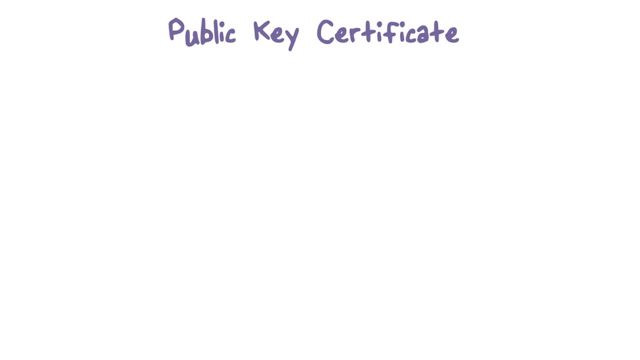 and a fake public key of his was being used. But then what can Bob do? Bob can send Alice another message saying that, hey, this is my real public key. but how could Alice tell That is, how could Alice tell that the previous key was a forgery? and 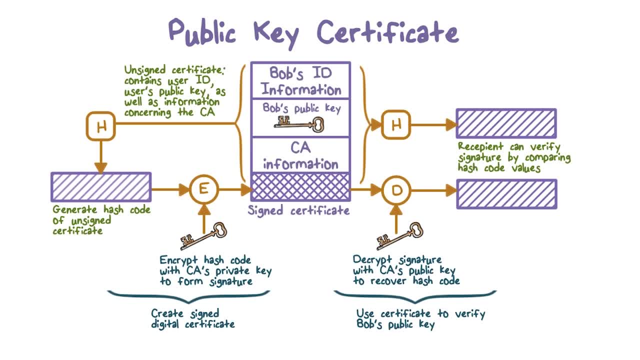 this key that Bob just sent is real. The solution to this problem of public key forgery is to use a public key certificate. In essence, a certificate consists of Bob's public key and Bob's information, such as the user ID- let's say his name and address, and so on. 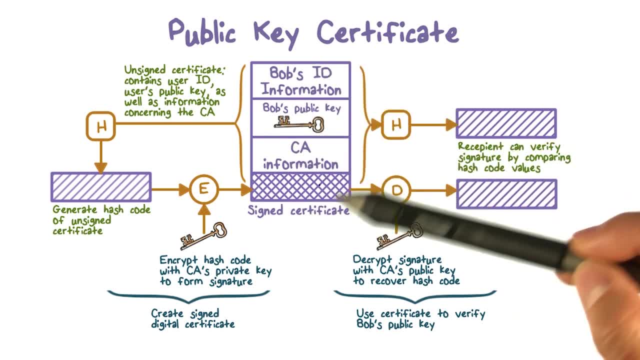 The certificate authority's information and the whole blog is signed Using the certificate authority's private key. The certificate can also include other information, such as the period of validity of this certificate, That is, for how long this certificate is valid for this public key. 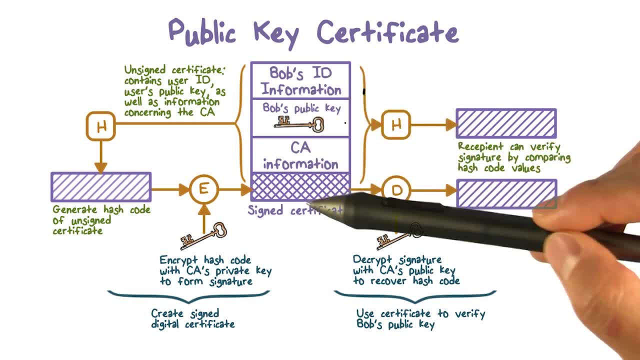 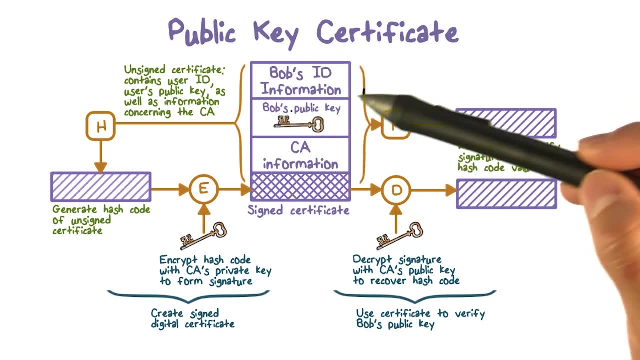 Say one year. Now let's see how certificate is created and how it is verified and how it is being used to distribute public key. Suppose Bob wants the certificate authority, CA, to create a certificate for his public key. Bob would contact the CA and provide authentication information. 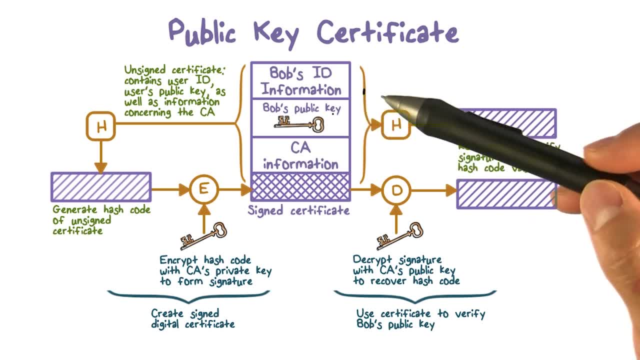 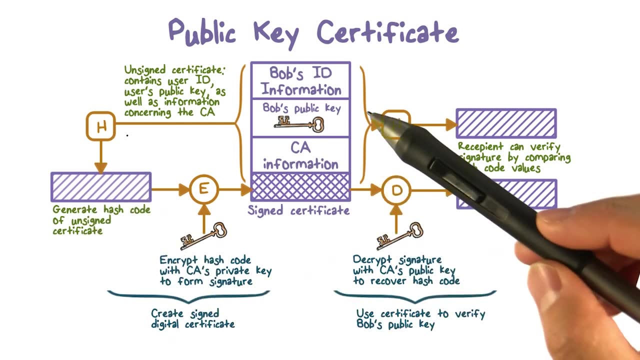 such as his driver's license and so on, And then he would send his public key to CA. The CA will then poops ID his public key and other information, such as the period of validity, together and then hash it, And then the CA will use his private key to sign the hash. 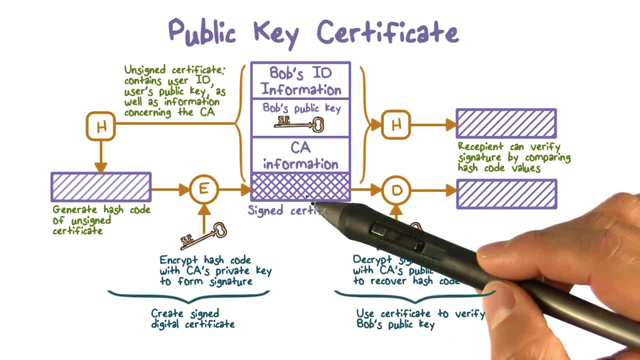 So that creates the certificate of Bob's public key. Now Bob can send this public key certificate to anybody, Such as Alice. When Alice receives this public key certificate, she can first extract the clear text information of Bob's ID, public key and other information. 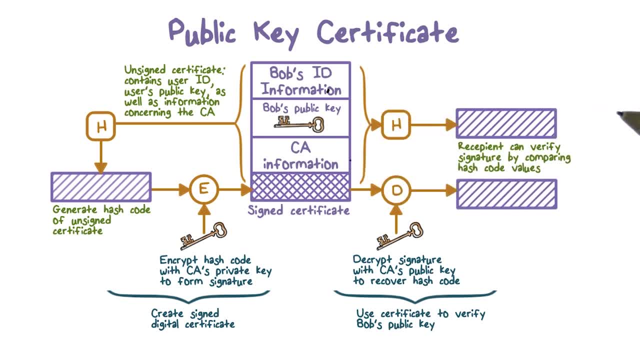 And then she will hash this data And then Alice would also use the certificate authority's public key to decrypt the signature or verify the signature And compare these two hash values. If they match, that means this public key has been properly signed by the CA.